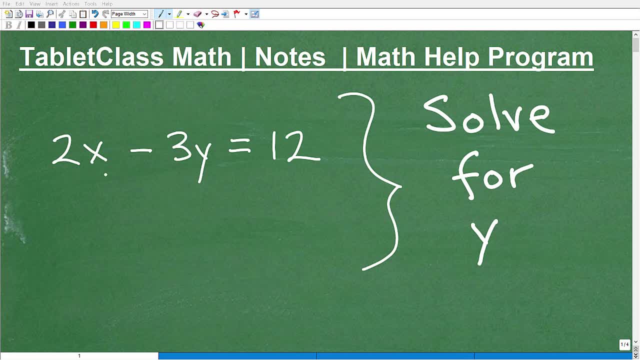 Okay, let's go ahead and solve for y in this equation. Okay, so we have 2x minus 3y equals 12. And our objective here is to rewrite this equation such that it's going to say y equals then whatever. Okay, so we're going to take this 2x, part these numbers and we're going to move everything over to this other side. We're going to have to do a few other steps, but we want to solve for y, or another way of stating this is to write this equation. 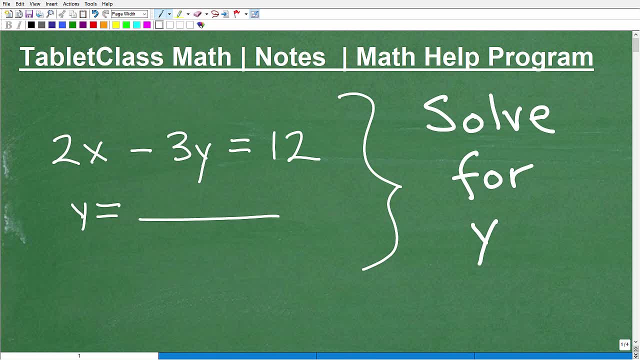 in terms of y. Okay, and y is just one of the variables in this equation. We have x and y And essentially the steps that we're going to take are going to be the same steps as if we were going to solve for x. But this is a critical algebra concept and skill that really trips up a lot of students, And it's absolutely necessary to be able to write equations in terms of different variables. When you have more than one variable in an equation, This comes up over and over. 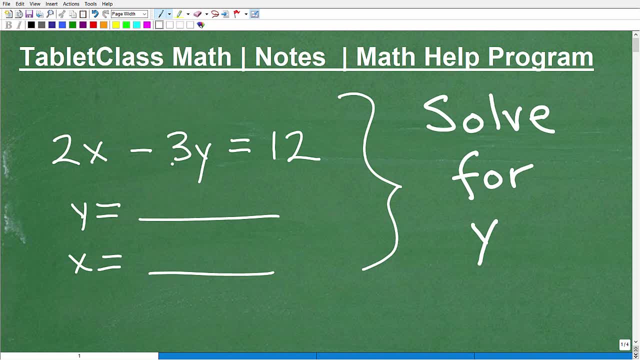 again in algebra. So hopefully you're going to stick around and learn this and master this. That's the whole objective of this particular video. But before we get into this problem, let me first go ahead and introduce myself. My name is John. I'm the founder of Tabit Class Math. I'm also a middle and high school math teacher And over many years I've constructed what I like to believe is one of the most robust online math learning programs there is. Okay, so I want to let you be the judge of that, But I'm going to leave a link to my math help program in the description of this video. 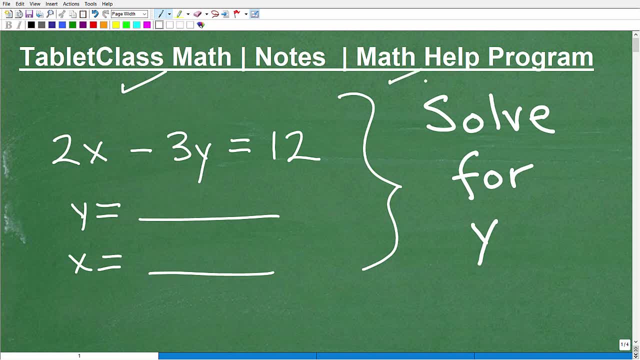 So, whether you need to take a full math course or you need help with the course that you're taking, my program just might be for you. Okay, it's all video based, super, super comprehensive, So if you like my teaching style, you're going to get my best work and explanation here. Now, one of the things I like to stress in all these videos is people don't realize the importance of math notes. Well, maybe I don't want to say everybody does, but it's critical. Okay, one of the things you need to really focus on is 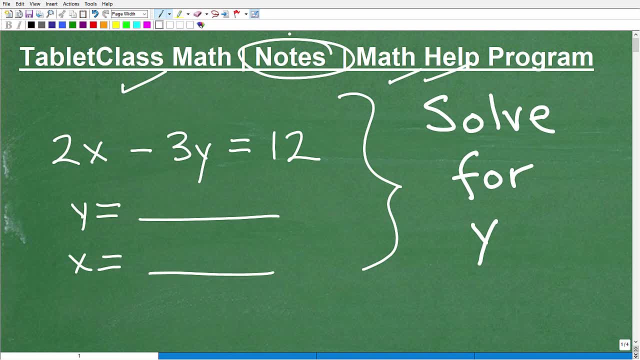 taking outstanding math notes. Okay, and that's a skill and it doesn't usually come easy to a lot of people. I know myself I had to really work hard at it. But it's just a rule of thumb: Those students who have great math notes typically have great math grades, and the reverse is true. If you are kind of inconsistent or disorganized or sloppy or don't really take note taking seriously, it's probably going to reflect in your grade. Okay, so this is after several, several 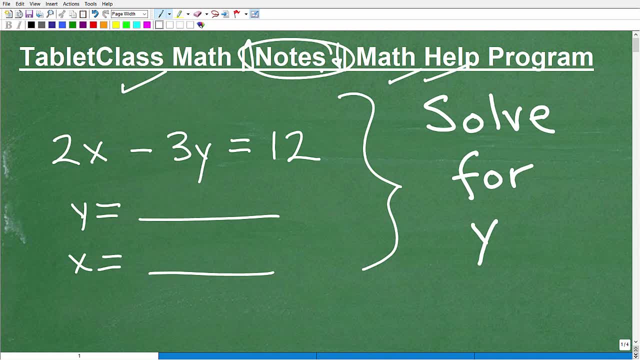 years of teaching math, you see these trends and they become kind of rules that you live by. But in the meantime, you need something to study from as you're improving your math notes, if that's if your notes aren't what they need to be. But I'm going to leave a link to my math notes in the description of this video, And those would include pre algebra, algebra one, geometry and algebra two and trigonometry. Okay, so the don't have anything to study from right now. you can get my math notes, but are extremely detailed and comprehensive. All right, so let's get into this. 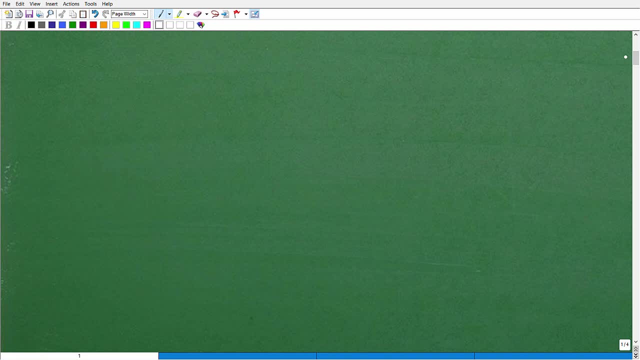 problem. And first I just want to explain why something like this is so important: this, this skill. So let's say I had 2x plus 5y equals nine, and maybe 3x minus 7y equals I don't know. let's say three, Okay, And we have some sort of system of equations. Now, if you haven't studied systems yet, you will be shortly Okay. so if you're looking at this video- because you're kind of doing this in math class right now- 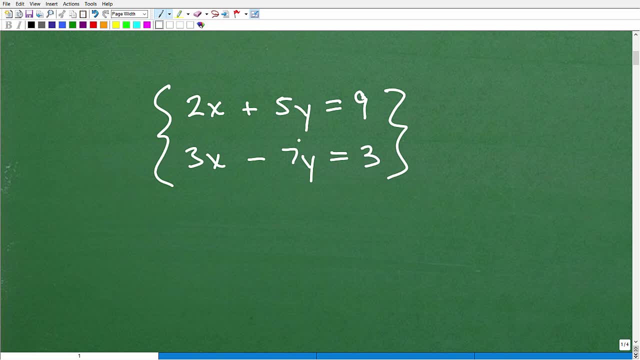 well, this topic of system is going to be coming right around the corner. Okay, But one of the ways we can solve this system is to use something called the substitution method. Okay, And it would. the substitution method basically requires us to take one of these equations and solve for one of the variables. So, for example, I could take the first equation and, let's say, solve for x, okay. or I could solve for y, or x down here, or y down here. In other words, I have to take this equation and rewrite it. 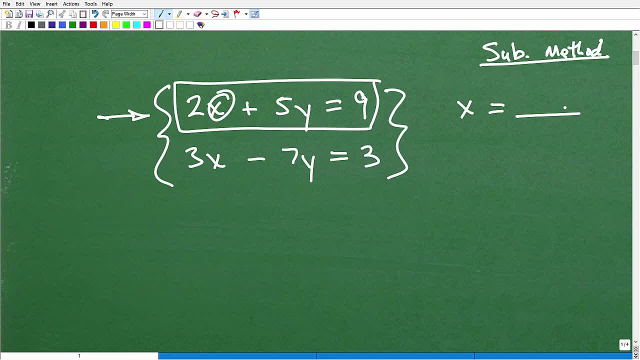 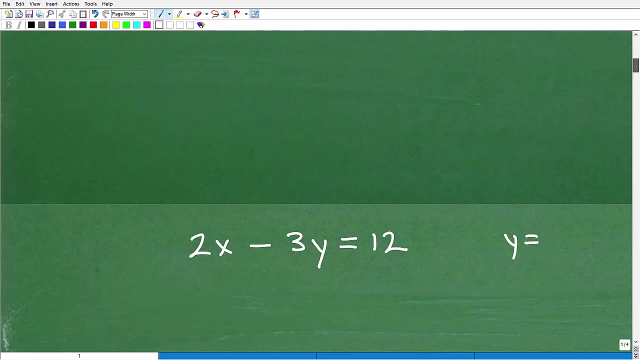 Such that it's going to say x equals whatever. Okay, and that's the skill that we're practicing in this particular video. Okay, And many students struggle with solving systems because they can't take this first step for solving for a particular equation. Okay, So that's what we're going to be doing. Obviously, I have an example problem, But let's start off with an easy version here. Okay, so here's: 2x minus 3y equals 12.. And 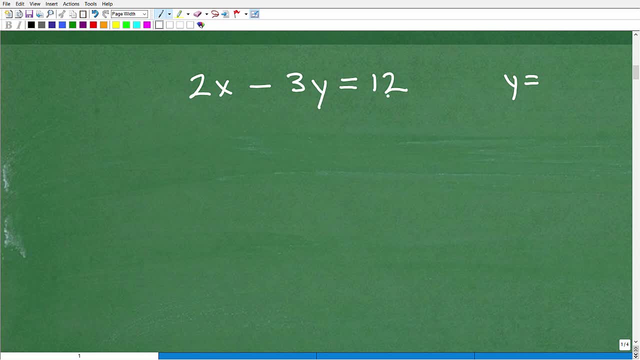 now, the first thing is you need to understand how to solve basic equations with single variable, what we call single, single variable, linear equation. So, for example, let's say I had 2x minus 3 equals 12.. So we'll just get rid of the y here for a second. Okay, So this equation, how would we solve this? Okay, so hopefully you're like: yeah, this is easy. What you would need to do- let me write that a little bit better- is: we have to add: 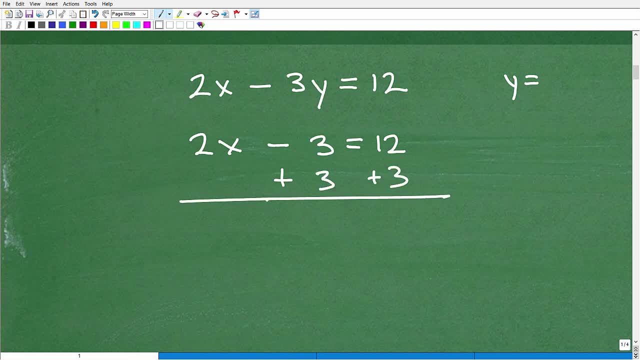 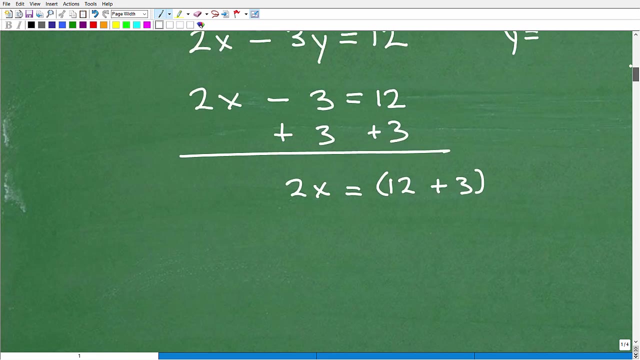 2x to both sides of the equation, And then we would go ahead and add down. we have 2x equals 12 plus 3.. And this time, of course, 12 plus 3 is 15.. But I'm gonna write it this way: 12 plus 3.. Okay, which course is 15.? And you'll see the reason why I'm kind of doing it this way in a second. And then here I'm going to divide both sides of the equation by 2.. So I get: x is equal to 12 plus 3, divided by 2.. 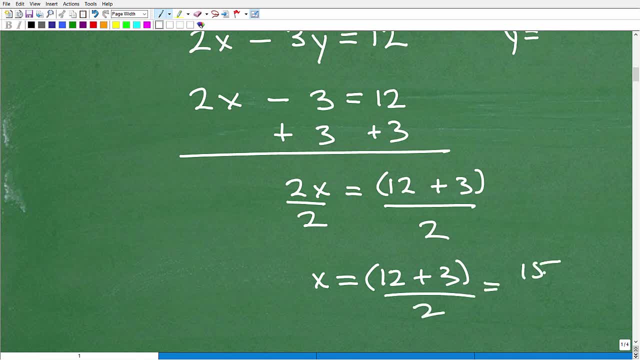 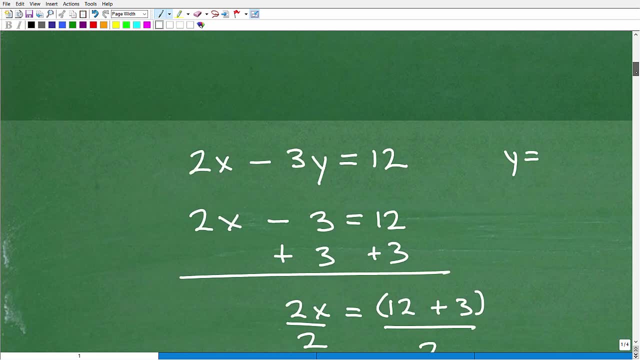 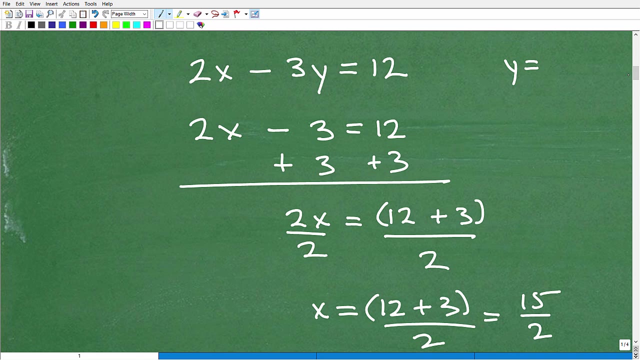 2, of course. 12 plus 3 is 15. so 15 over 2 is what x is equal to. okay, so no big mystery. hopefully you know your. this was pretty easy and you're like, yeah, that's all right, i understand that. well, if you understand this, then you're going to understand, um, how to, how we solve for a particular 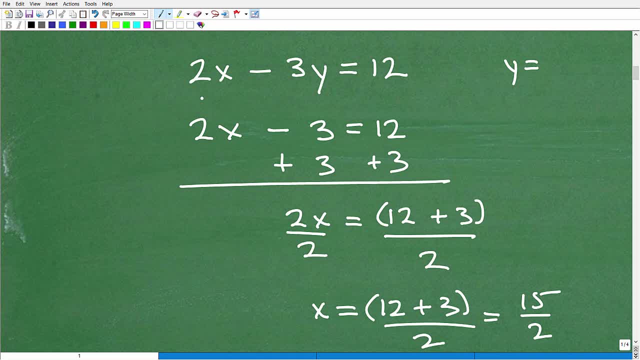 variable. okay, so i'm going to get to solving for y, but let's first solve for x, because we already have this kind of set up right now. okay, so the way you solve for a variable when there's more than one variable in an equation, is to identify the variable that you're solving for. we're going. 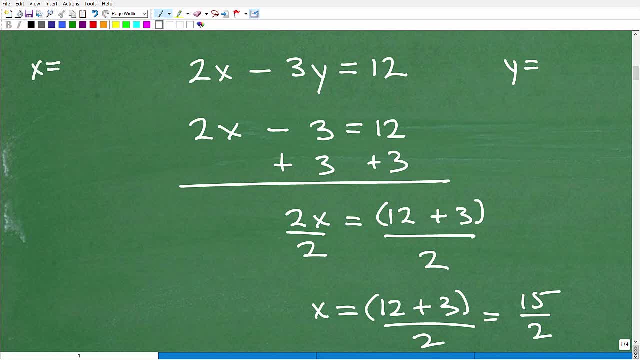 to solve for x first, and then i'm going to finish up by solving for y. okay, so let's say i said: solve this variable for x. well, i look at my equation right here and i'm going to say, okay, x, all right, this x here. this is the only thing i'm going to conceptually think of as a variable. in the words, i'm going to: 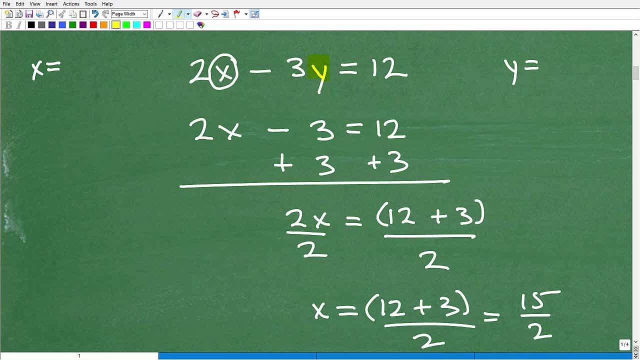 think of this y as a number, just for the time being. okay, so any number you want, doesn't make a difference. let's say it's one. okay, so this will be three times one, or it could be two, three times two, six, doesn't make a difference. this, this becomes like one unit, one value. okay, so let's. 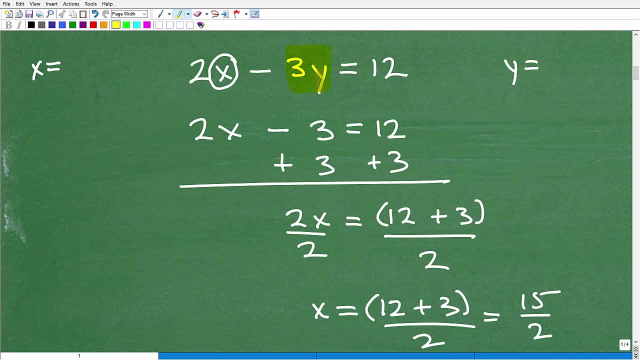 say: uh, for the time being, where we're just going to think of y, is one all right. so to solve for x, we're going to think of x as a number, okay. so let's say, for the time being, for x, i would literally just do the what i just did right here. okay, this, this, basically. 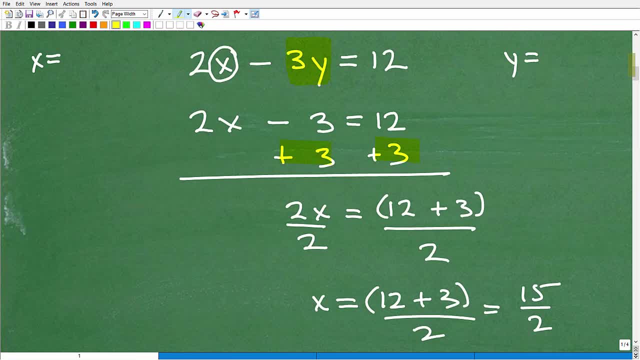 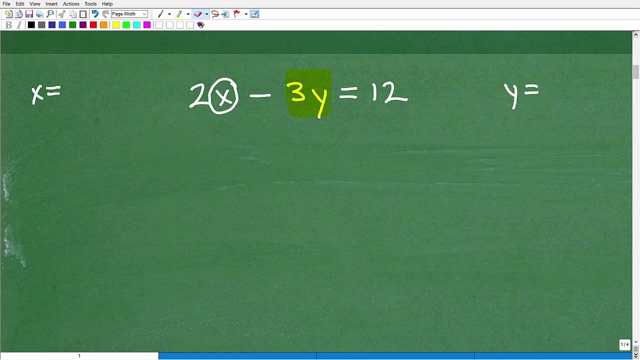 this same step, but now, okay, i'm just kind of follow through what i did. let's go ahead and do this, all right, and now i'm going to solve for x, but and then we're going to go back and finish up by solving for y, okay, which was our original problem, but i just solved for x and i was 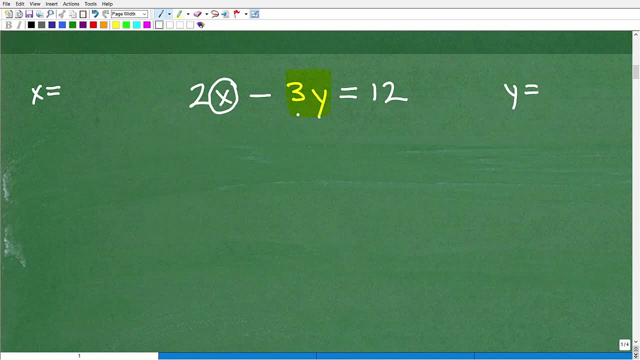 thinking this as a number. okay, so let's solve for x right now, and what we're going to do is: okay, three, y- i'm thinking of x- is only as a variable, so this i'm just going to think of as one number. okay, all right, anything just in your, whatever works for your brain, just be like: okay. 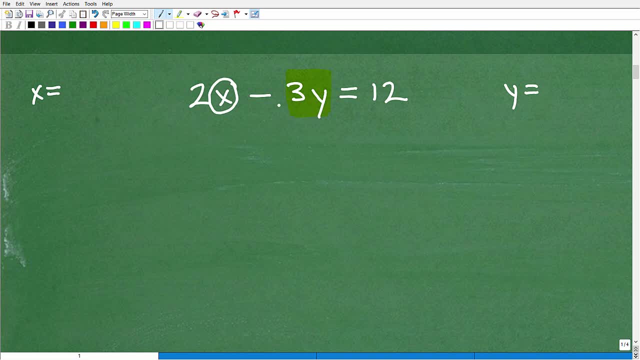 three times a number is some number. it doesn't make a difference. whatever that value is, i need to move it to the other side, remember? if this was just three, i would add three to both sides of the equation, right, but it's not three, it's three y. okay, so it's just some other number, but we have 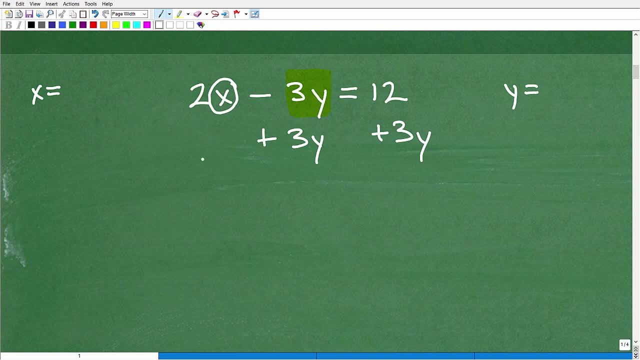 to include the y. okay, you understand. so, because we're taking the same equation, solving steps, all right, we're only treating this x- because we're trying to write this in terms of x- as a variable and we're treating this y as any particular number. okay, so now i want to add down. all right, i'm going to get 2x. all right, by itself is equal. 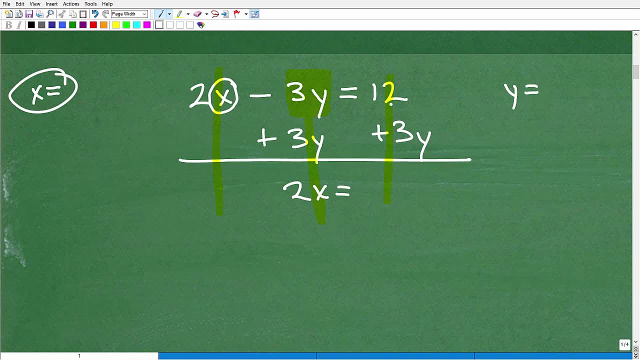 to negative 3y plus 3y, that's they cancel each other out, right? so now i have 12 plus 3y, 12 plus 3y. okay, now you can kind of understand why i was right and it says 12 plus 3. 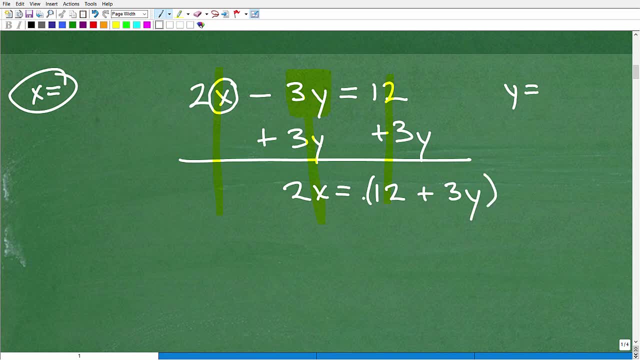 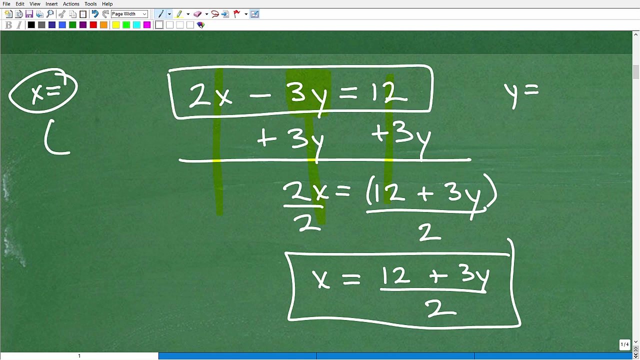 in my previous example, and i'll put parentheses around that. and now to solve for x, i'm simply going to divide both sides of the equation by 2. so x is equal to 12 plus 3y divided by 2. all right, so what we just did here is we rewrote this equation in terms of x. 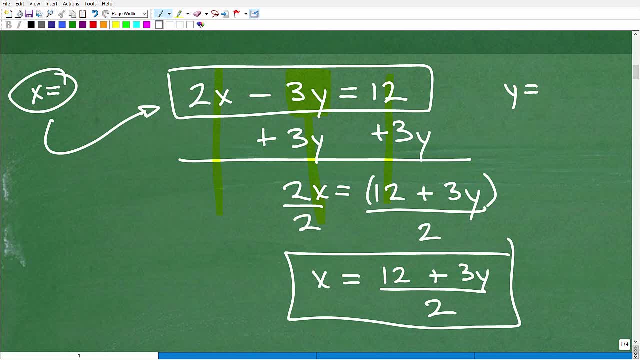 okay, that's how you would state that. so the instruction would be: hey, write this equation in terms of x or solve this equation for x. okay, and this would be the answer. okay, so here's my y, and so if you feel like you understand this, okay, let's go ahead and finish up by solving for y. 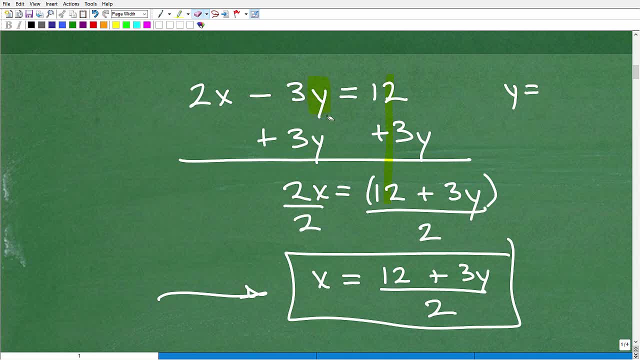 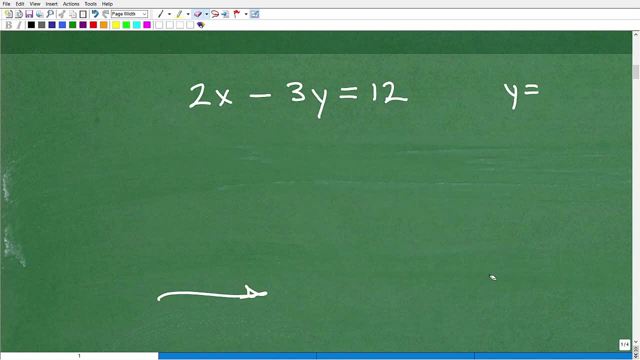 and that was our original objective. of course, i was going to do it for you, but i want to train you up so you can do it right. so you should go ahead and give it a try and see if you can do it. try if you feel like you uh could do this problem. so rewrite this equation in terms of y. in other, 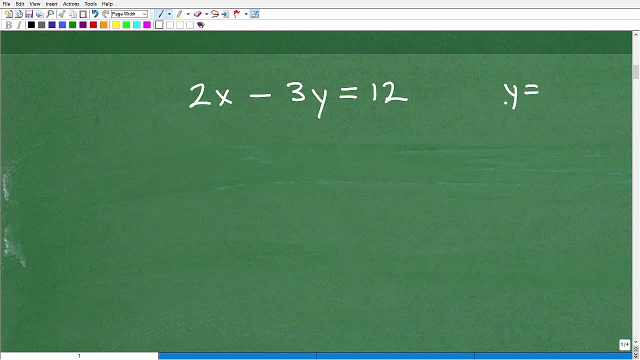 words: solve for y. okay, so we don't want to see the solution. uh, just, you know, uh, right now you might want to pause the video and try it, but i'm going to go ahead and solve it. so we're going to be thinking of y as the only uh variable, okay, so x 2 times x is like 2 times 2 could be 4. this is: 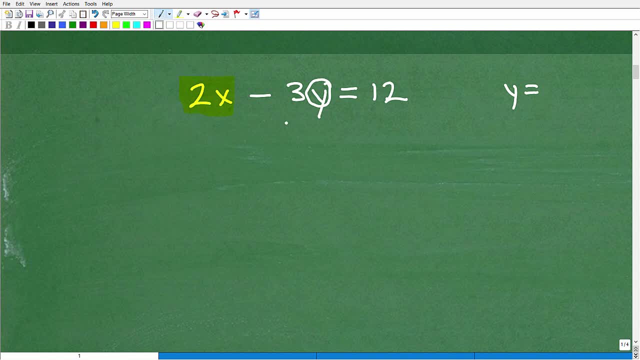 some value, okay, some number. so if i have, let's say, 2 minus 3y equals 12. you're confused on what to do. you'll be like, oh yeah, the first thing i'm going to do is i'm going to subtract 2 from both sides of the equation. okay, and that's what. 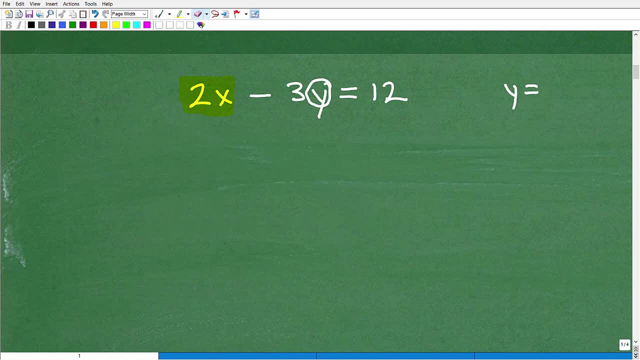 we need to do here, but it's not 2, it's a 2x. so i'm going to subtract a 2x from both sides of the equation and now, when i add down boop, boop, boop, okay, i have positive 2x minus 2x. that's of course. 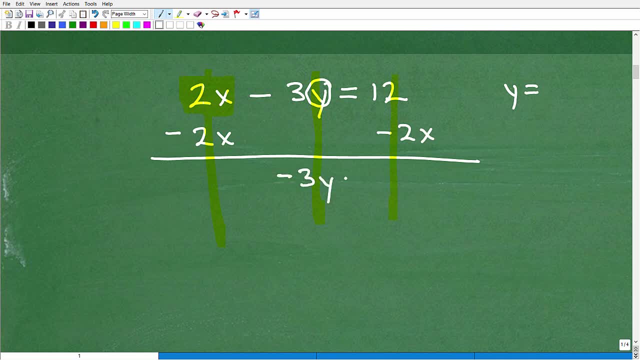 zero and i have this negative 3y equals. now here i have 12 plus a negative 2x. we could just write this like so: 12 minus 2x, and now this is a difference. it's always a good idea to put grouping symbols in there. okay, like so and to. 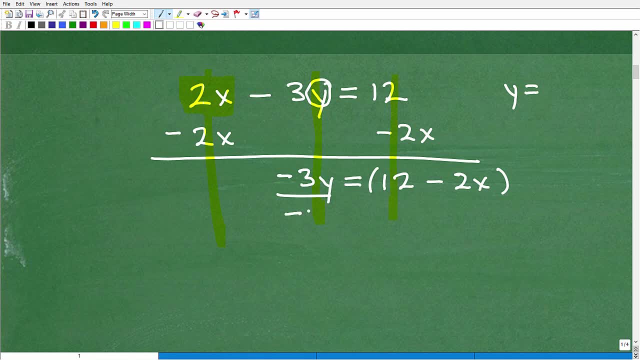 solve for y. now all i have to do is divide both sides of the equation by negative 3 and you have y is equal to 12 minus 2x. let's put some parentheses around that over negative 3 and we are done. okay, we'll give ourselves a smiley face and we got this right. give yourself. 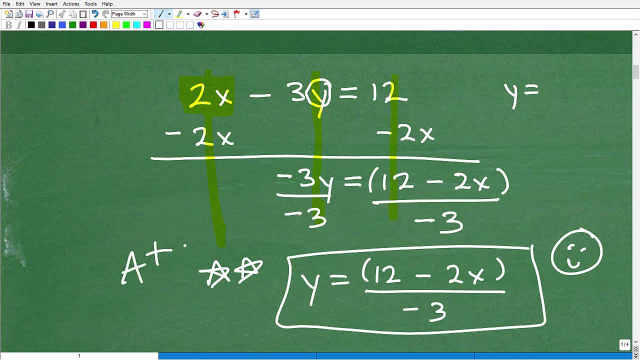 some stars, a plus, whatever makes you feel good. it's always nice to see those things on your. you know feedback from a test or quiz and all that good stuff. of course, as a math teacher, you really enjoy giving those things out. you hate to go like minus 10, minus 10. i used to hate that. 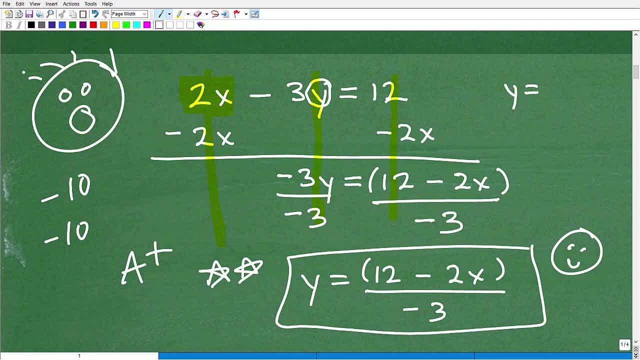 because then people's reaction would be like this, and then it would just be like, oh, tears and listen. all that could be avoided, right? how do you avoid situations like that? well, you got to be paying attention, you got to work hard. learning math is not going to happen, uh, automatically. 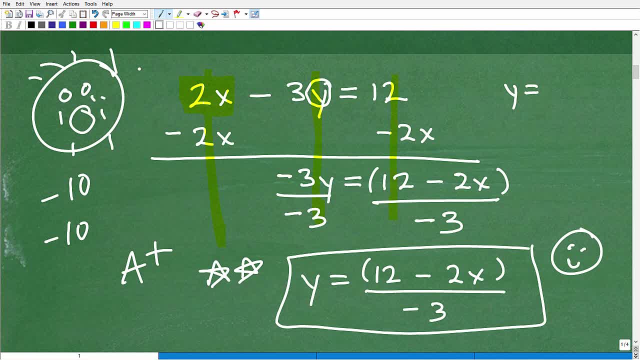 okay, it's something you have to work at, and if anyone's telling you anything different- like, oh, there's a shortcut, you can, you know? uh, any a program out there, or or whoever you might be listening to, say, oh, you could just do this, you don't need that. like always looking for the path, 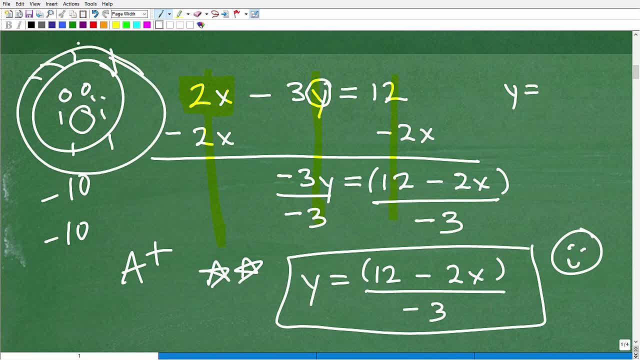 least resistant or shortcut. i'm telling you that's going to always end up being a shortcut to this right. there's only one way to learn math, and that is to work hard, practice, practice, practice. okay, you need to have all the fundamental skills. no taking, you need great instruction, okay, so 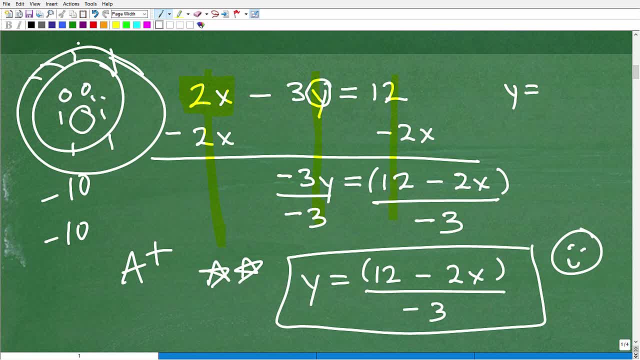 hopefully you're getting that from your teacher. if not, you can look for other teachers out there that you better understand. maybe it's myself or somebody else, but you have to help yourself. okay. but i can tell you right now, absolutely unequivocally: you can learn mathematics, no matter.